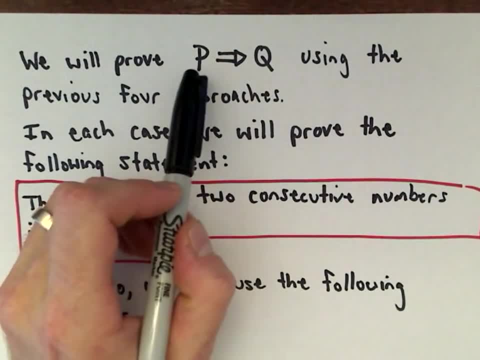 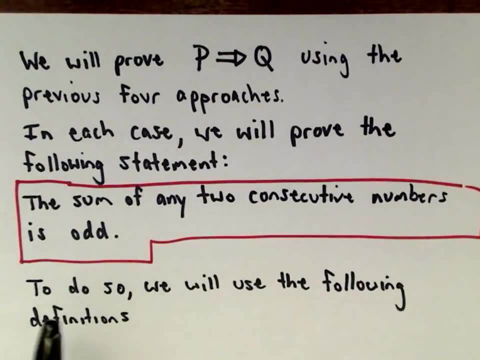 direction. So we're going to prove one of these if-then statements- if P, then Q- And we're going to use the four approaches. we just mentioned, those different types of proof techniques. So what we're going to prove in each case is we're going to prove the following: 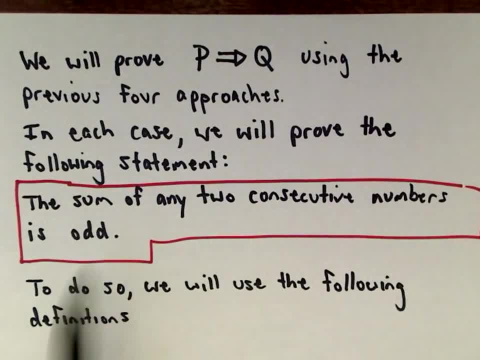 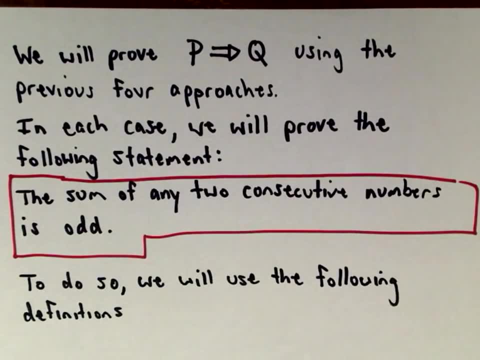 It says the sum of any two consecutive numbers is odd. And again, not a mind-blowing result by any stretch. So write: 3 plus 4 is odd, 4 plus 5 is odd, 5 plus 6 is odd, etc, etc, etc. And to do that, well, we're going to. 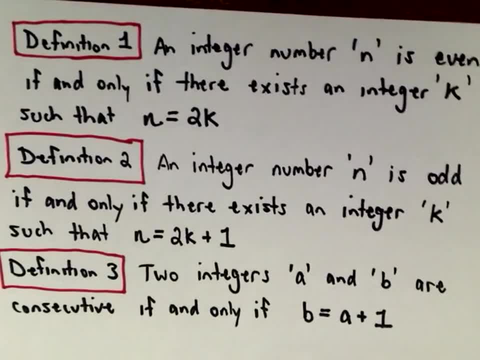 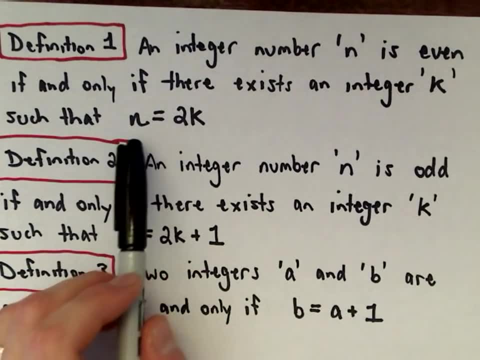 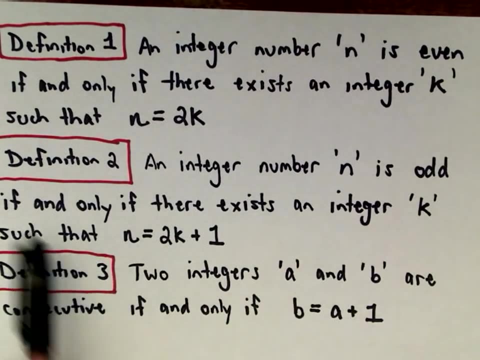 use some definitions. So definition one: so an integer number n is even if, and only if, there exists an integer k, so that we can write that number as n equals 2 times k. Definition two: An integer number n is going to be odd if, and only if, there exists an integer k such 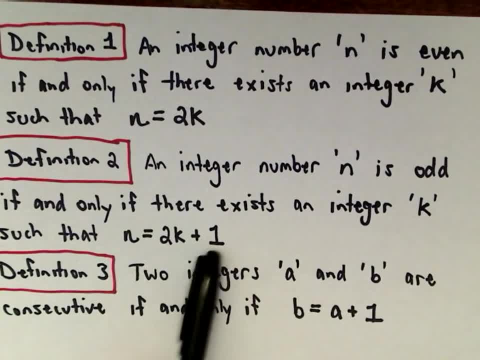 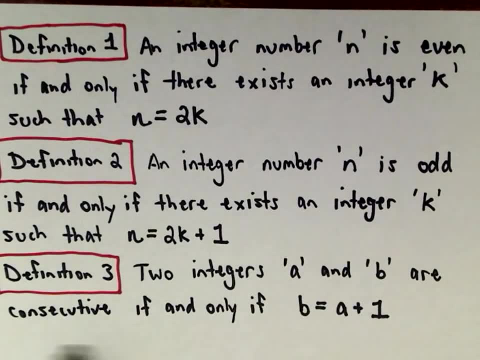 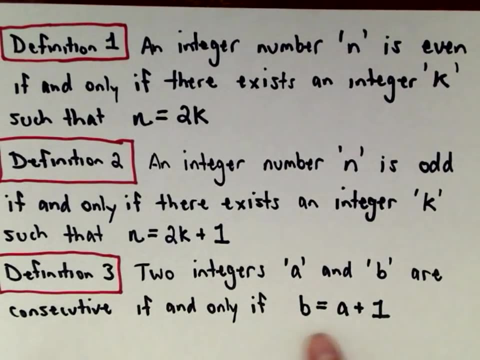 that we can write n as equal to 2k plus 1.. That's going to be the definition of an odd number And definition three. Two integers, a and b, are going to be consecutive if, and only if, b equals a plus 1.. So one number, one of the numbers, is one larger than the. 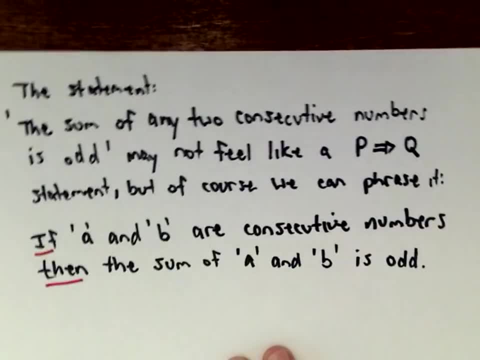 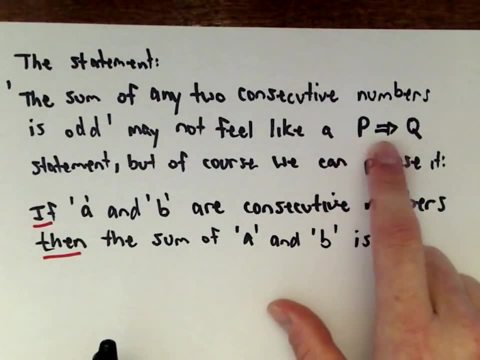 other one. right, That's what they're saying. Okay, So this statement- the sum of any two consecutive numbers is odd. it may not at first glance feel like one of these if-p-then-q statements, but of course you could rephrase this slightly and we could put the if-then. 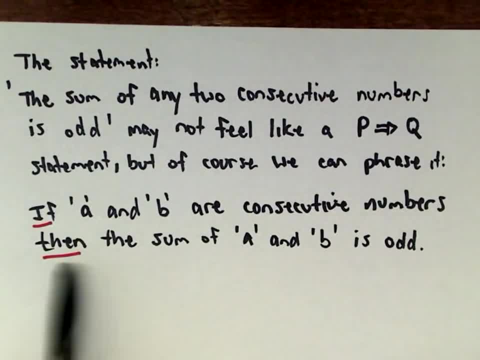 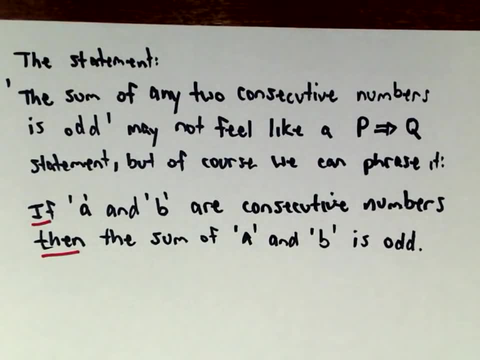 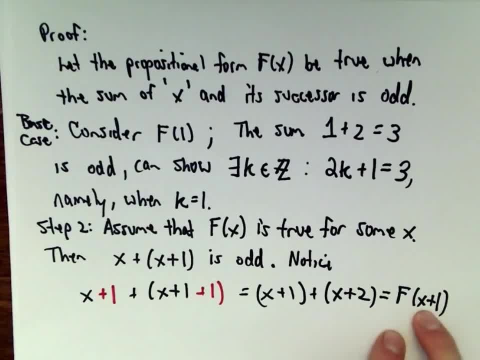 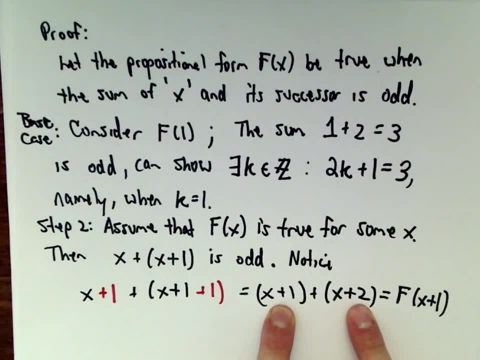 Because we said our propositional statement, we take whatever number that's next to our f, that's inside of our f, and we take its successor and we add those together. So this is going to be the propositional statement: f of x plus 1.. 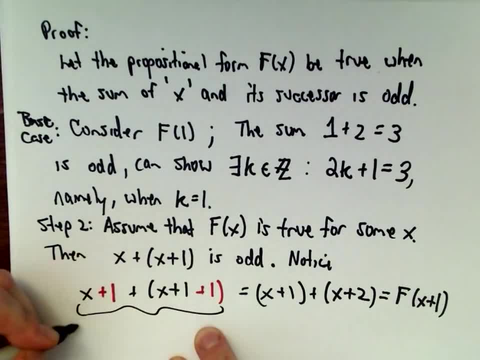 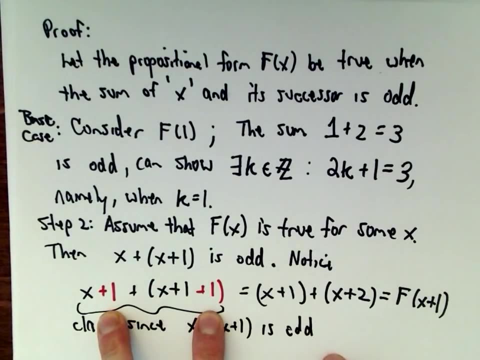 And we can certainly claim. so our claim here is that, since x plus x plus 1 is odd, what did we do? Well, we really just added 2, right, We added 2,. we added 1 plus 1.. 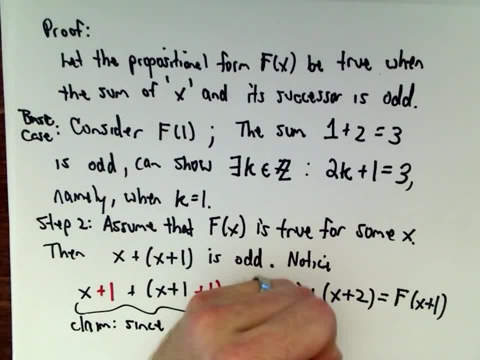 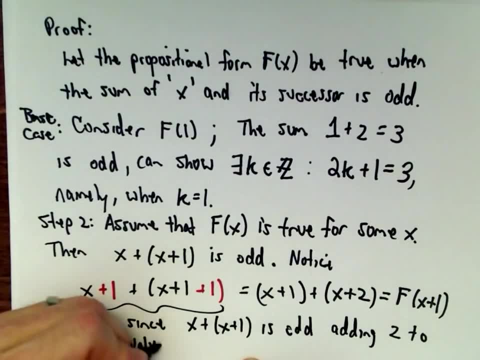 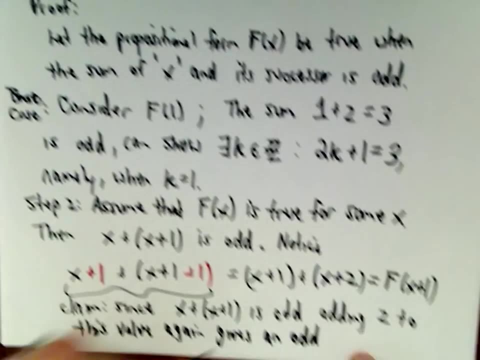 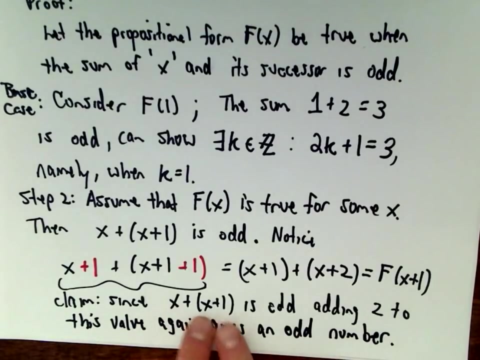 So since x plus x plus 1 is odd, adding 2 to this value Again gives an odd number. This again gives an odd number, and that would be proof complete. So since x plus x plus 1 is odd, well, if we add 2 to that, it's still going to be odd. 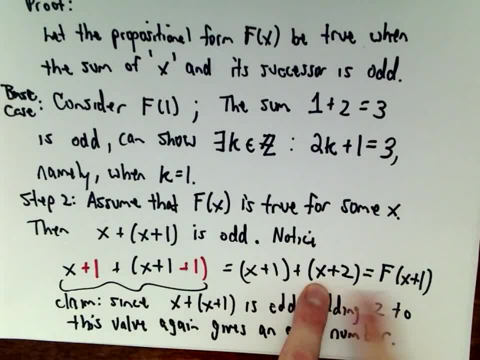 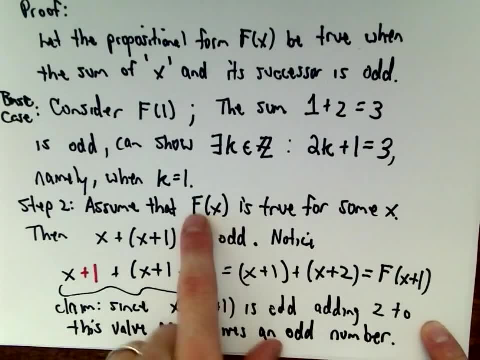 But when we write x plus 1 plus x plus 2, that's going to be our next propositional statement. So, assuming that f of x is true, we've now justified And true in the sense that it's going to be. 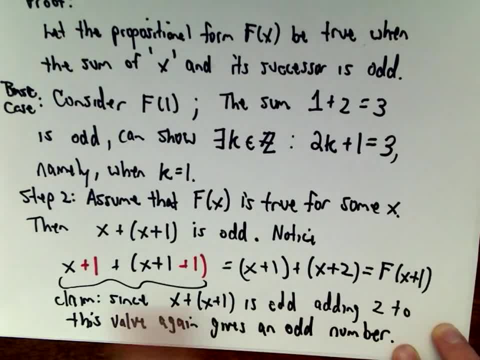 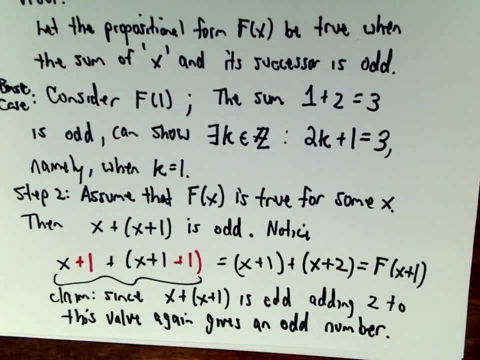 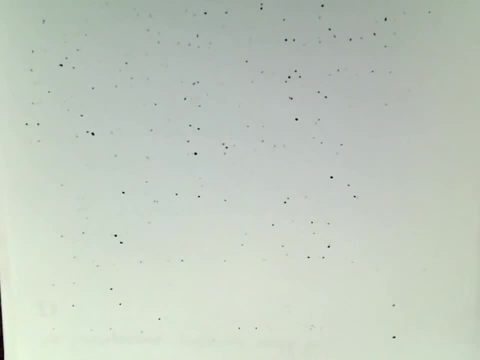 This statement is odd. We've now shown that its successor is also odd. So that would be a proof by induction. So that would be our general step here. Last but not least, let's look at proof by contrapositive. Okay, so proof by contrapositive. 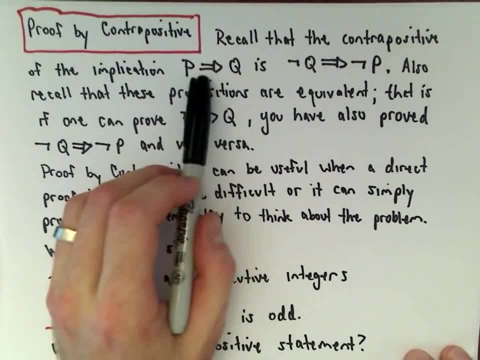 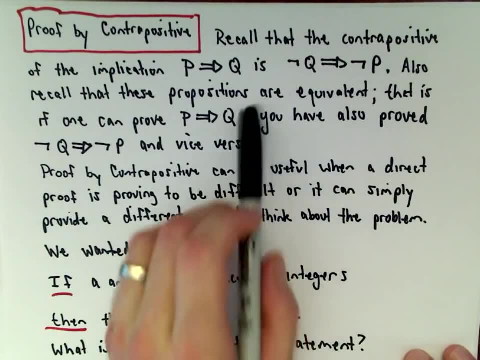 So the contrapositive of the implication fp then q. the contrapositive of that is: if not q then what? If not q, then not p. And these propositions are equivalent. And what that means is that if you can prove the implication fp, then q. 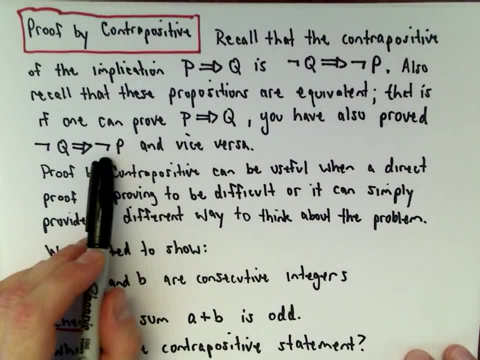 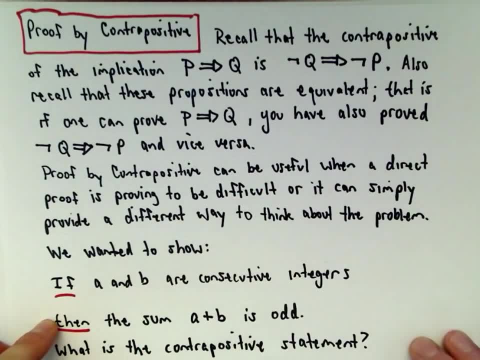 you've also proved the implication: if not q, then not p and vice versa. So, just as I've got written here, proof by contrapositive can be useful when a direct proof is either a little bit difficult or just sort of by flipping the statement around a little bit. 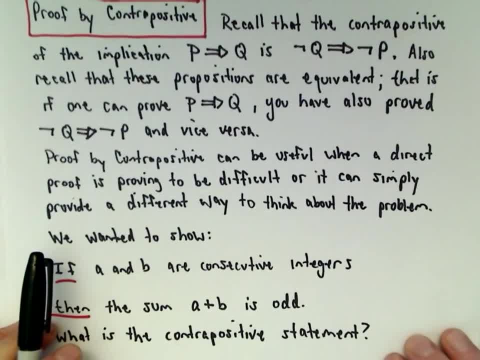 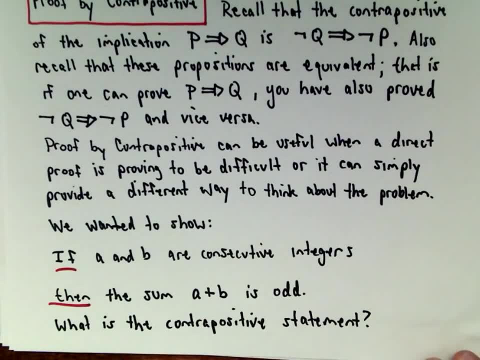 it sort of gives you a different way to think about the problem. So again we wanted to show if a and b are consecutive integers. the sum a plus b is odd. So think about that for a second. What would the contrapositive of that be? 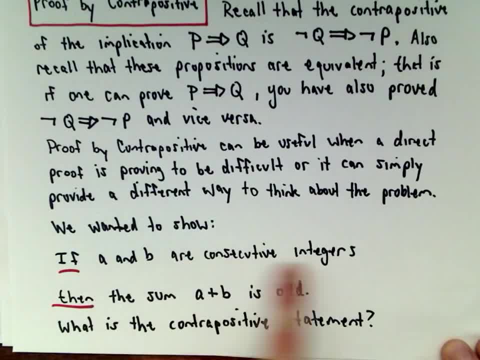 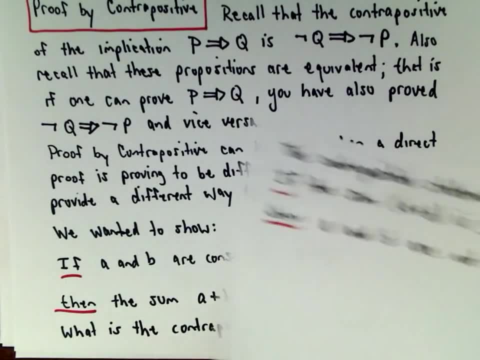 Well, okay, so this first, if that's our statement p. So if a and b are consecutive integers, then the sum a plus b is odd. So that's our statement q. So now we flip them around and we negate, So our q goes first. 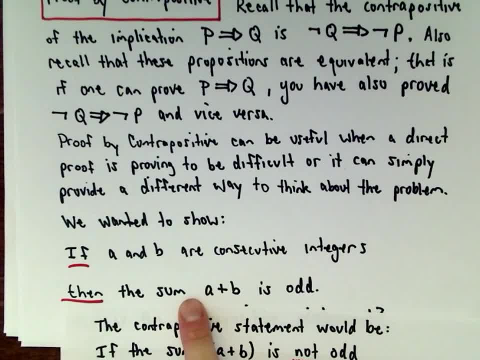 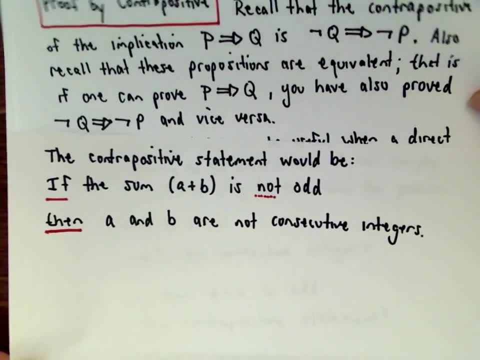 q goes first and we put a not in front of it, We're negating it. So if the sum of a plus b is not odd, then a and b are not consecutive integers. That's going to be our contrapositive. 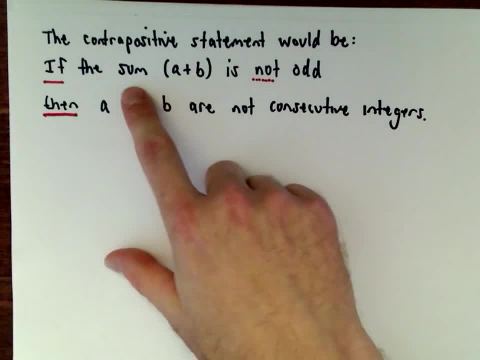 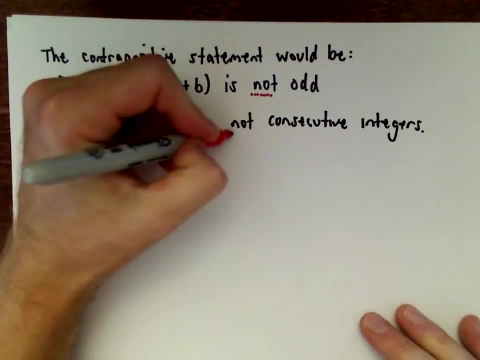 And that's what we're going to try to. we're going to try to prove this if-then statement. Okay, so this is going to be our contrapositive statement now, And I've got not underlined there once, Let's underline: not in there again. 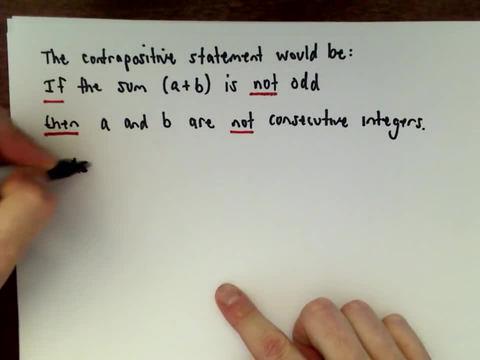 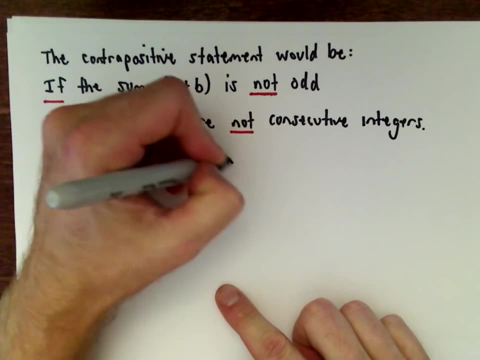 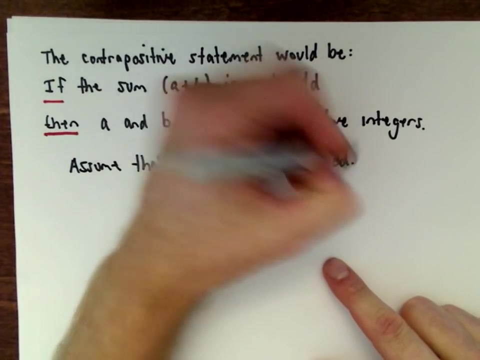 Okay, so, okay, so let's prove this. So we're going to assume. so we're going to assume that the sum of a plus b, so the sum a plus b, is not odd. That's our assumption. So that means there does not exist. so there's our little exist statement. 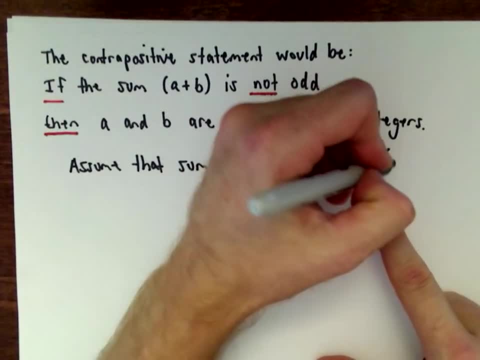 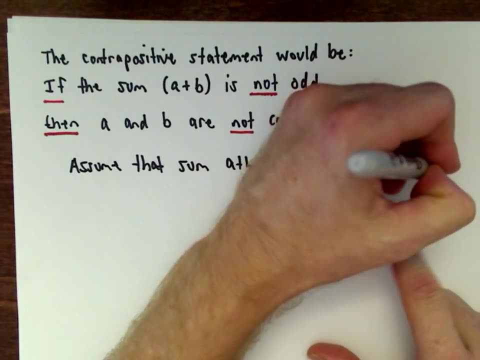 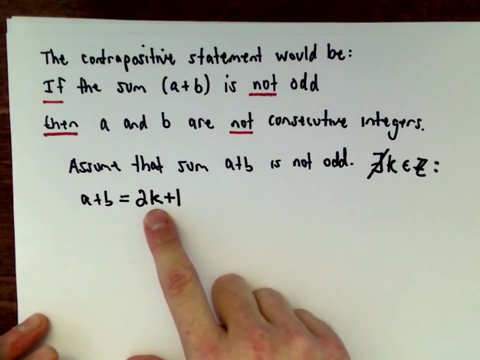 And we put a line through it that means there does not exist an integer k. So there does not exist an integer k Such that we can write a plus b as 2k plus 1.. This integer k does not exist. Okay, so because if it did right, a plus b would be odd. 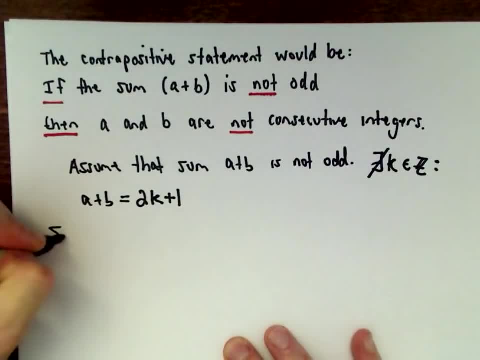 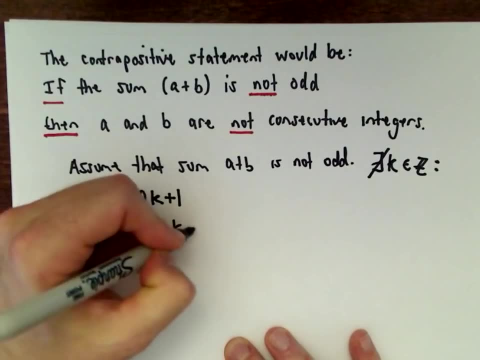 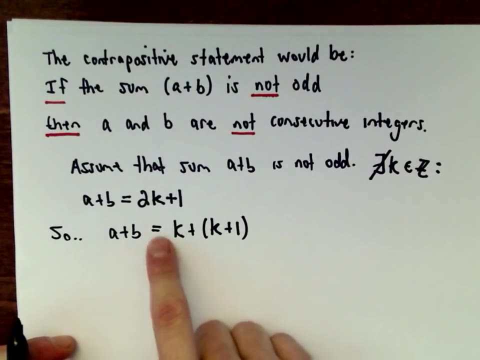 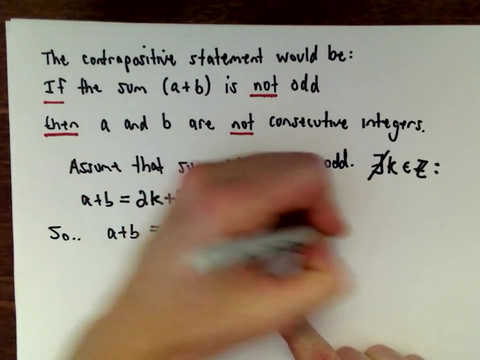 So this, this does not exist. So well, we can again rewrite this. I could write 2k plus 1.. I could write that as k plus k plus 1.. So this statement- A plus b equals k plus k plus 1- does not hold for any integer k. 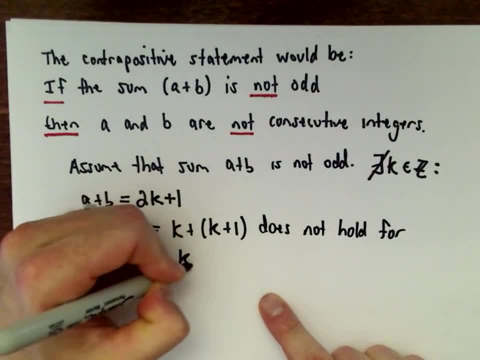 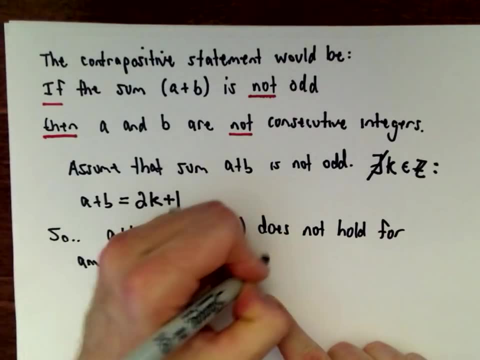 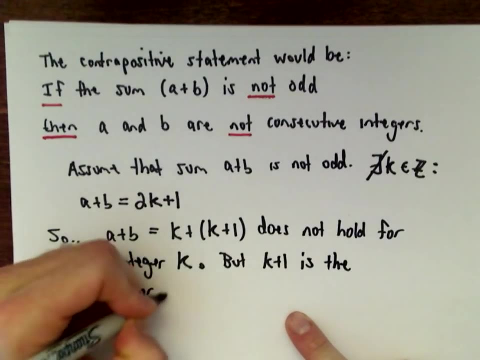 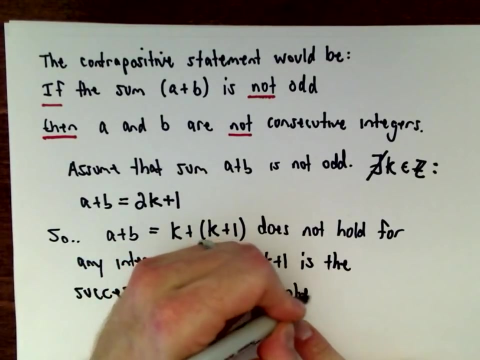 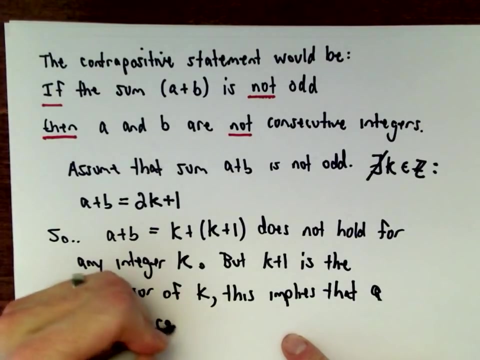 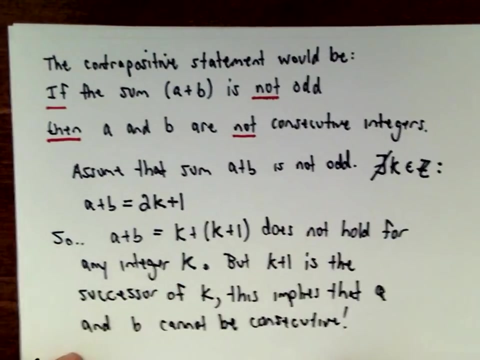 And. but notice, you know, since, but since k plus 1 is the successor Of k, This implies, This implies that a and b Cannot be consecutive, Right? so since? since we can't write a plus b as some integer, k plus k plus 1.. 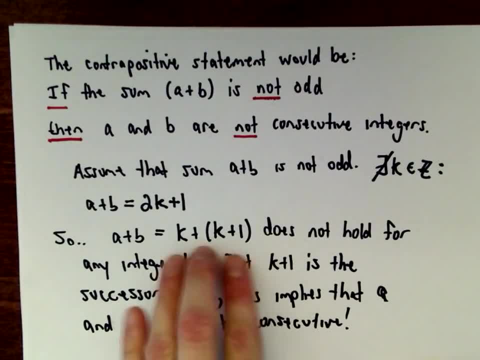 Right. so, since, since we can't write a plus b as some integer, k plus k plus 1. Right. so, since, since we can't write a plus b as some integer k plus k plus 1. Right, if, if we could do this.